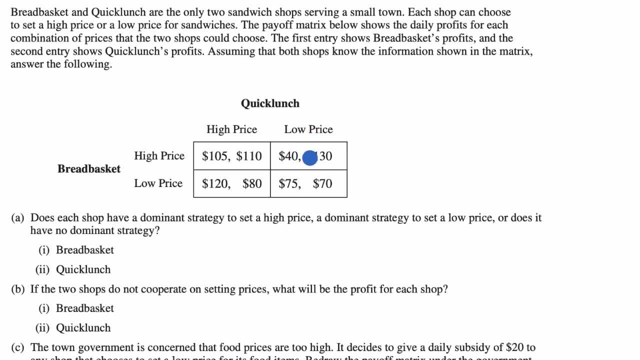 we can see what are the profit of either when bread basket charges high prices or bread basket charges low. So with that out of the way, let's try to answer these questions. Does each shop have a dominant strategy to set a high price, a dominant strategy to set a low price? 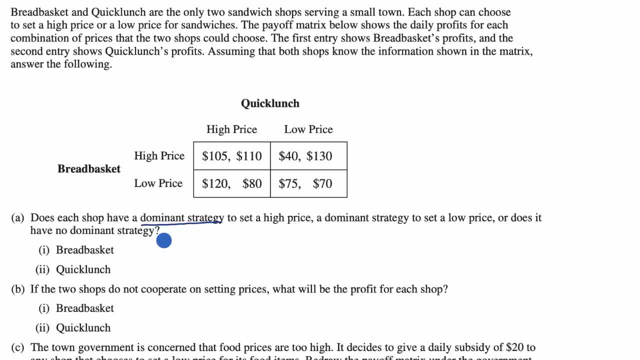 or does it have no dominant strategy? So pause the video and try to figure that out. And just as a bit of a hint or a reminder, a dominant strategy is a strategy of regardless of what the other player does. you would still be better off to make that choice. 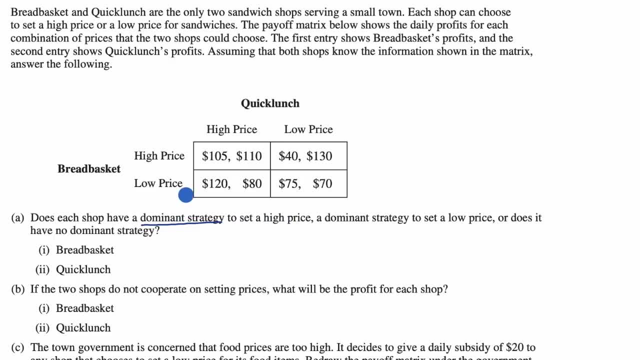 So a dominant strategy of setting a high price would be: regardless of whether the other player decides to set a high or low price, a high price would always make sense for you. So pause the video and try to see if you can answer that. 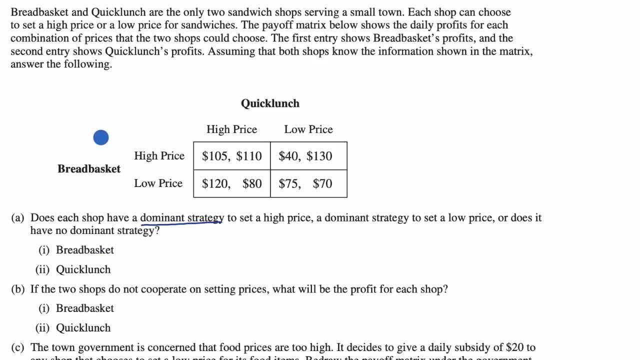 All right, now let's see what bread basket's situation is here. So if we think bread basket, of course, can either choose to go high or low, Now if quick lunch goes high, what should bread basket do? Well then we are in this column, over here. 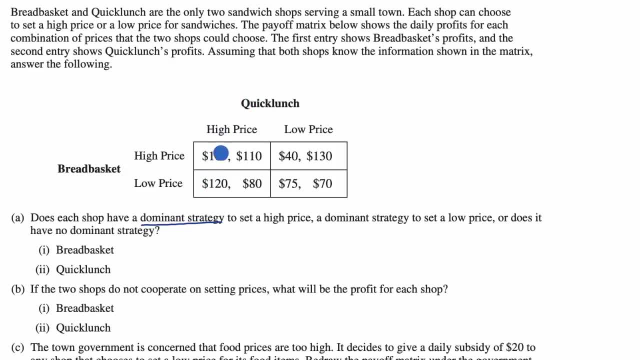 and these two numbers are for bread basket. And so if quick lunch goes high, if quick lunch goes low, What should bread basket do? Well then, we are in this column over here, And these two numbers are for bread basket. And so if quick lunch goes high, if quick lunch goes high, 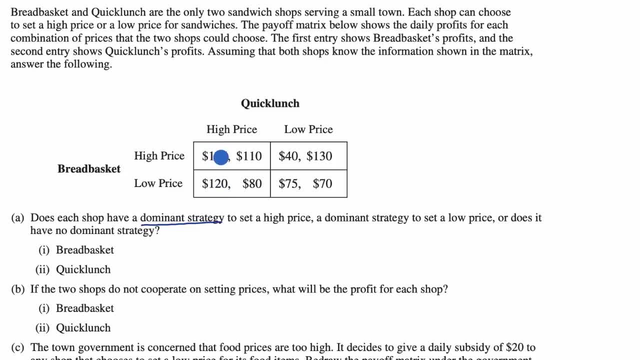 then bread basket could go high and charge 105, or it could go low and charge 120.. So if quick lunch goes high, bread basket should go low. So let me write this: quick lunch, quick lunch. If it chooses to go high, then bread basket should go low. 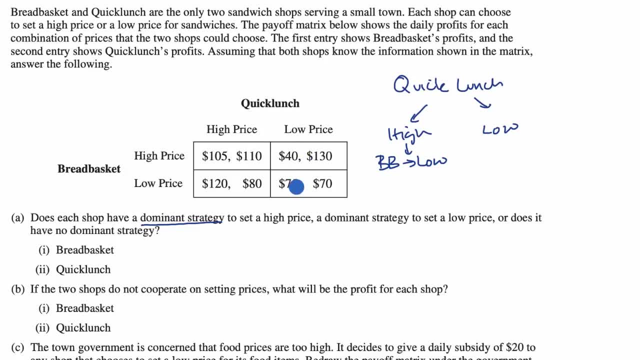 Now what happens if quick lunch chooses to go low? Well, if quick lunch chooses to go low, the two options for bread basket are either $40 of profit per day if they have a high price, because a lot of their business would go to quick lunch in that situation. 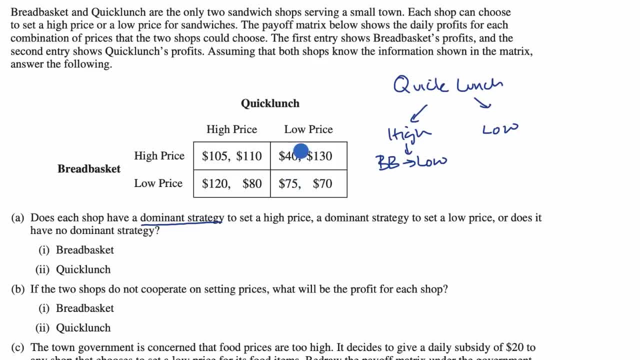 or they could go low price and make $75 per day. So even if quick lunch goes low, it still makes sense for bread basket to go low. So bread basket goes low. So we see that bread basket, no matter what quick lunch does. 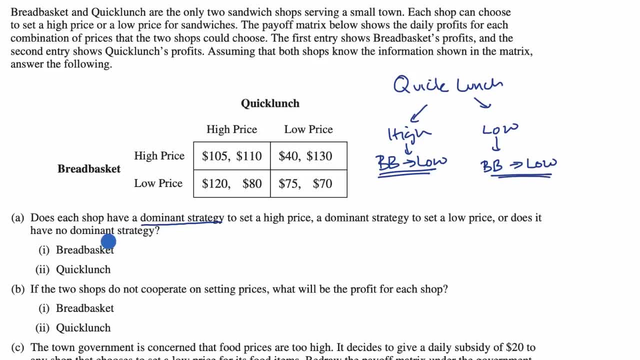 it makes sense for bread basket to go low. So bread basket has a dominant strategy to set a low price. So the dominant dominant strategy to set- let me write that a little bit clearer- set low price. All right, now, quick lunch. 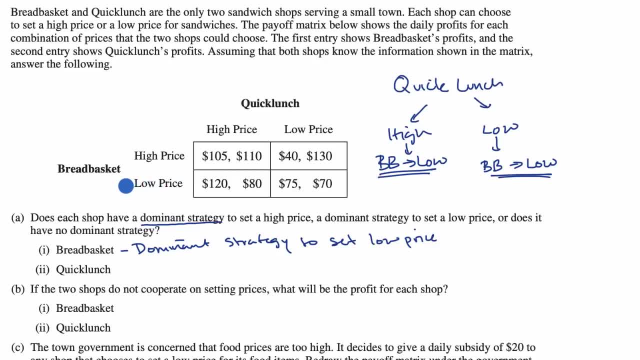 So we could do the same type of analysis based on what bread basket might choose to do. So if we see, okay, if bread basket goes high, what should quick lunch do? Well, let's see Then, quick lunch should. so if bread basket goes high. 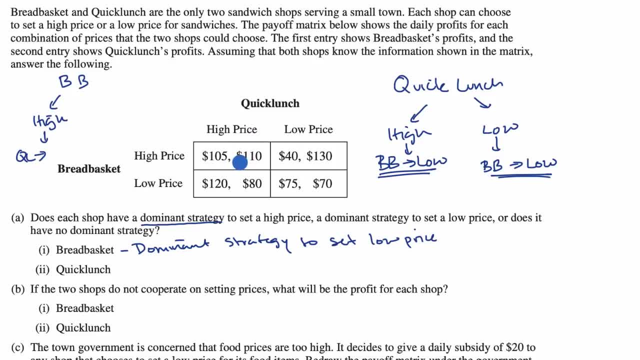 quick lunch. should it go high or low? So it would have an option of $110, or it would have an option of $130.. So if bread basket goes high, quick lunch is better off going low. So let me write that down. 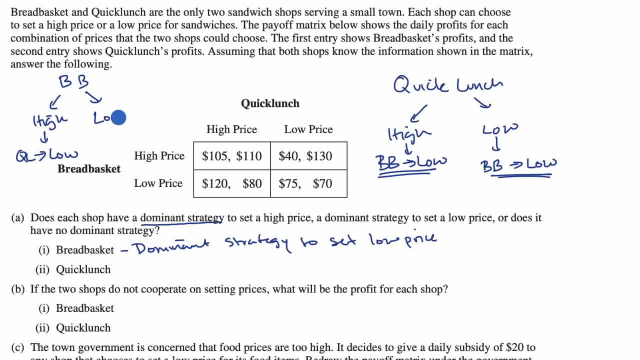 Quick lunch should go low. And if bread basket goes low, what should quick lunch do? So if bread basket goes low, quick lunch can either make 80, if it goes high, or 70, if it goes low. So in this situation, if bread basket goes low, 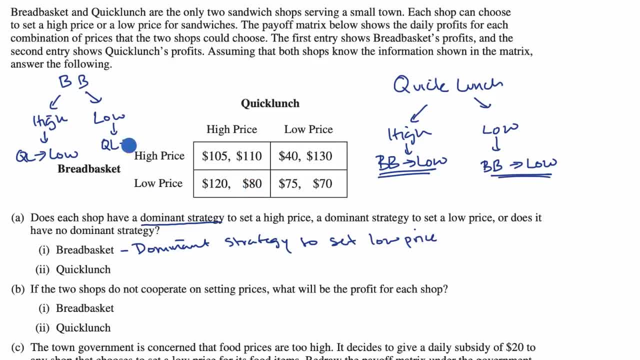 it makes sense actually for quick lunch to go high and make the 80. So quick lunch would go high. So quick lunch has no dominant strategy. It doesn't make sense for them to always go low or always go high, regardless of what bread basket is doing. 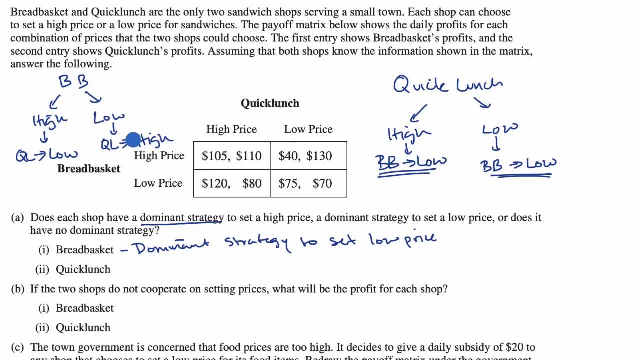 Depending on bread basket. it might make sense for them to go low if bread basket goes high or high if bread basket goes low. So no dominant, dominant strategy. If the two shops do not cooperate on setting prices, what will be the profit for each shop? 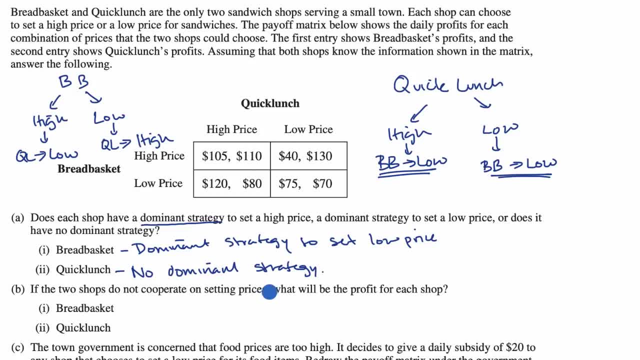 Well, actually, just pause the video, See if you can answer that before we work through it. Well, we already know that bread basket has a dominant strategy to set a low price, So bread basket is gonna go low regardless. So we're going to end up in this row right over here. 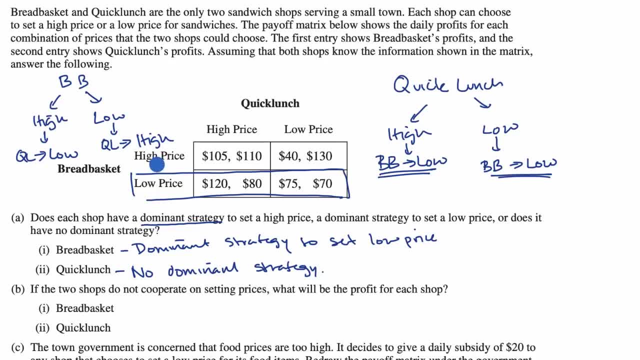 And if we are in that situation where bread basket goes low regardless, we know that it makes sense for quick lunch to go high, because they can either make 80 or 70. Well, they're gonna go high, and so we're going to end up in this column right over here. 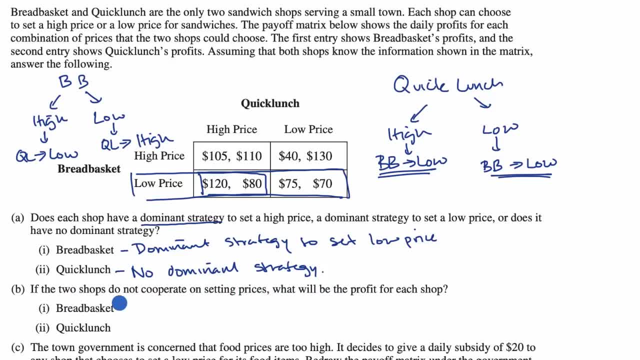 So if the two shops do not cooperate on setting prices, the profit of each shop would be: bread basket would be making $120 a day and quick lunch would be making $80 a day. And this is a Nash equilibrium because on its own, 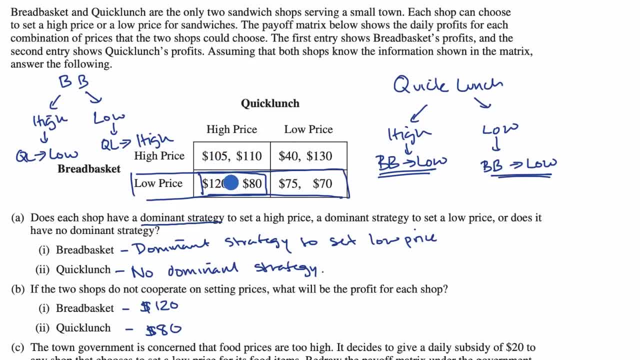 no firm can change its decision. It can't change its decision to optimize its prices more, Because if you are in this cell right over here, quick lunch can't change bread basket's decision. So quick lunch could say: I'm either gonna make 80 or I'm gonna make 70.. 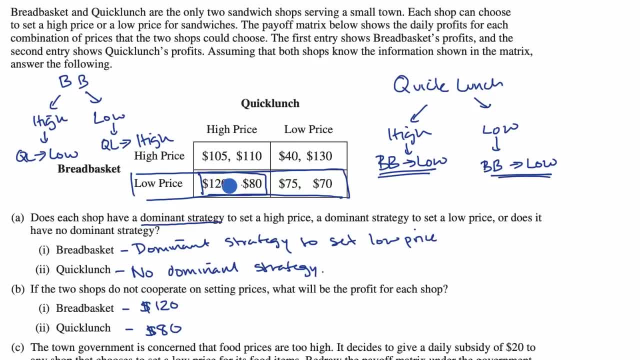 So it wouldn't make any sense for them to switch away And then bread basket. they can't make the decision for quick lunch. They can say, hey, we're either gonna make 120 or we're gonna make 105. And so since we can't change what quick lunch is doing, 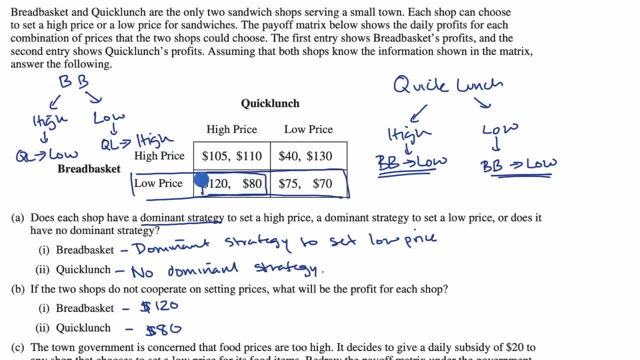 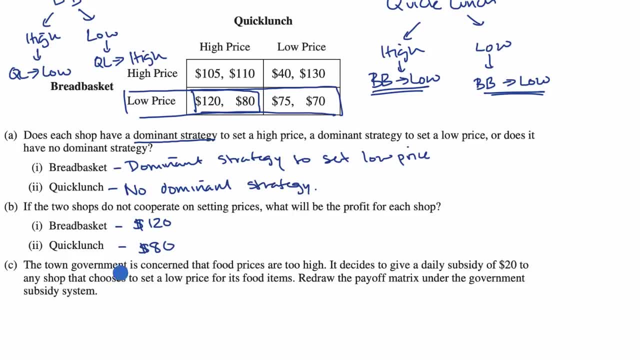 well, of course we're gonna choose to make 120.. So people will stay in this bottom left cell. We're in Nash equilibrium, All right. so the next part- they ask us or they tell us, the town government is concerned. 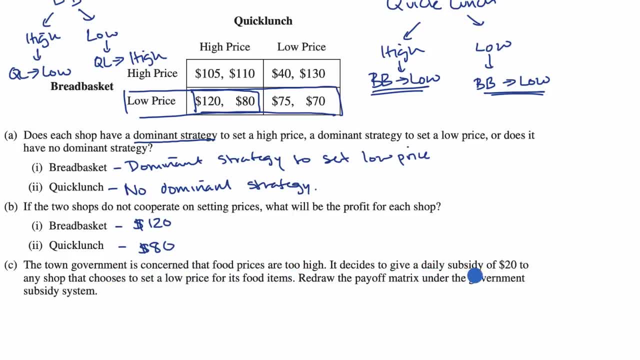 that food prices are too high. It decides to give a daily subsidy of $20 to any shop that chooses to set a low price for its food items. Redraw the payoff matrix under the government subsidy system. So, like always, pause this video and go through that exercise. 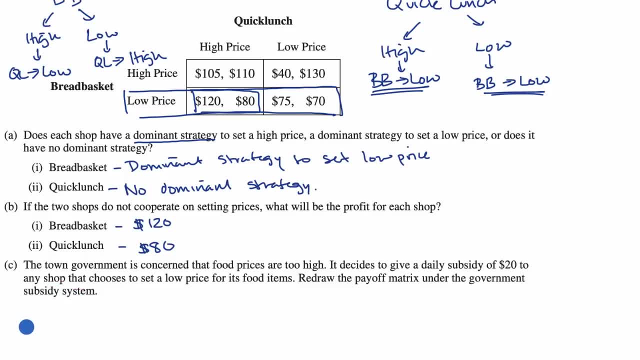 It'll be interesting. All right, now, let's do this together. So we have bread basket. I'll try to write bread. Actually, let me draw my little matrix first. So it's a two by two. So almost done with my matrix. 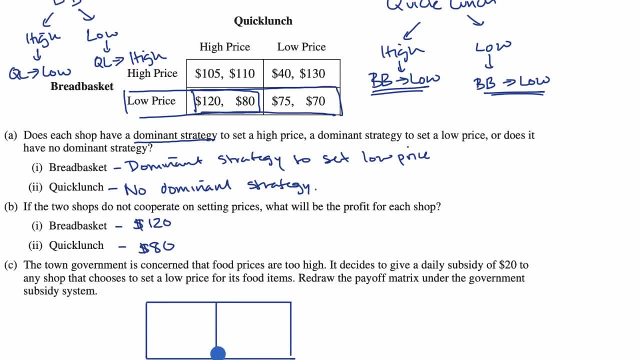 And one more. All right, that wasn't near the middle. There you go right around there. It's still maybe there, And then we have that there, And then we have high, low, high, low, And then you have quick lunch. 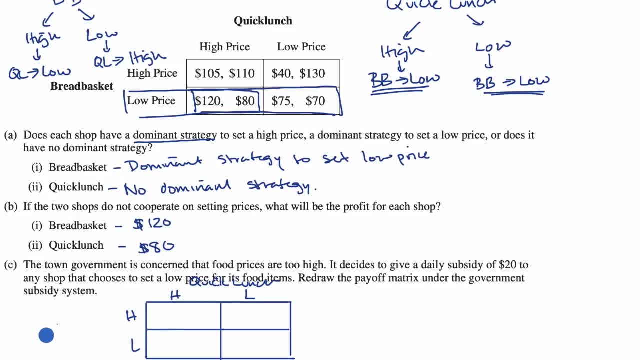 If I were actually doing this in the test, maybe I'd write this a little bit lower, so it's a little bit neater. And then this is bread basket And let's see it's giving a daily subsidy of $20.. So we can just do that. That adds to the profit of a firm that is selling at low prices. So if they're both at high prices, they're not going to be able to get that subsidy from the government. So we're still going to be at 105 and 110. 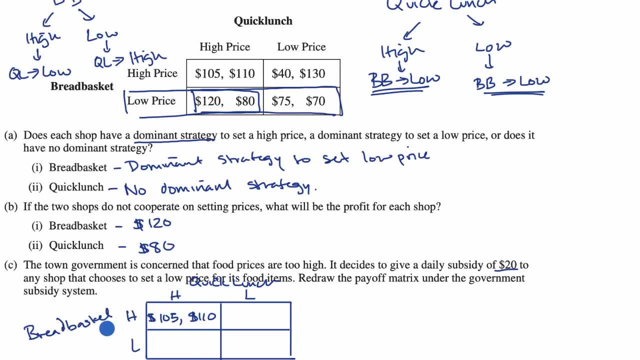 for bread basket. So bread basket and quick lunch respectively. Now, if bread basket stays high in this situation, well then they're still only going to make $40. But in this situation, right over here, quick lunch is going to get a $20 subsidy. 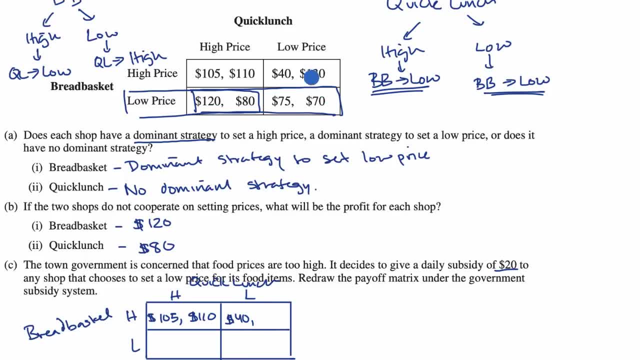 because they are choosing to go low. So they're going to make 130 plus 20.. So I'll write that in a different color, So I'll put that in and I'll put this in red. So 130 plus 20, they're going to make $150,. 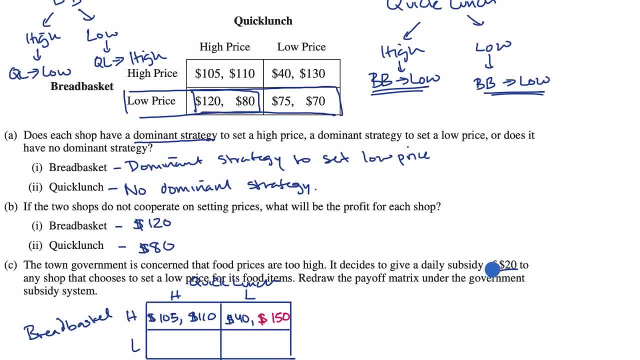 because they're choosing to go low. So they're choosing to go low. they're choosing to go low price here. That's what qualifies you for the subsidy. And in this situation, if Breadbasket goes low price, they're going to make 120,. 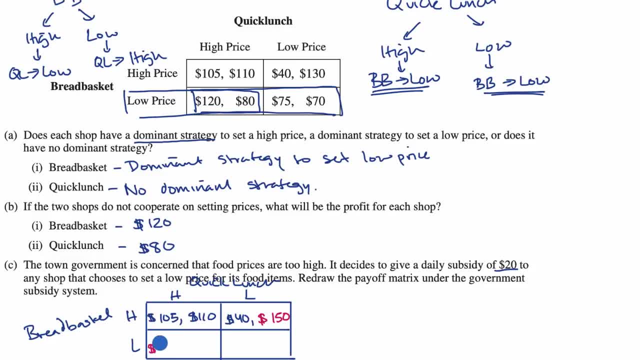 what they would have made in that situation plus 20. So this is going to be 140.. But this is a situation where Quick Lunch is charging a high price, So they're not going to get the subsidy, so they're still going to make $80. 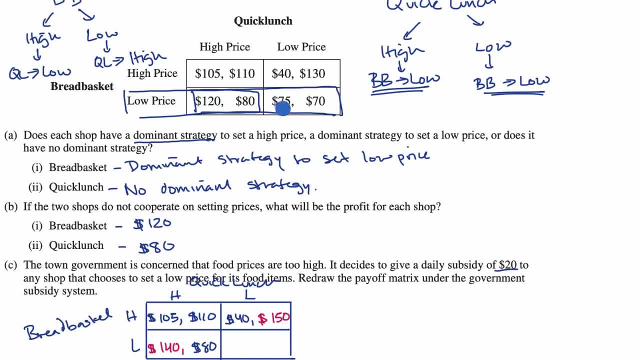 And then this cell is both of them charging a low price, so they're both gonna get $20 more than what you see right over here. So Breadbasket would make $95, $95. And Quick Lunch is going to make $90. in this situation, 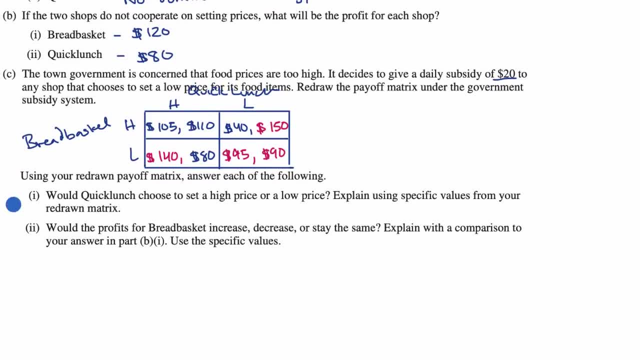 And let's see they ask us more questions. They say, using your redrawn payoff matrix, answer each of the following: Would Quick Lunch choose to set a high price or a low price? Explain using specific values from your redrawn matrix? 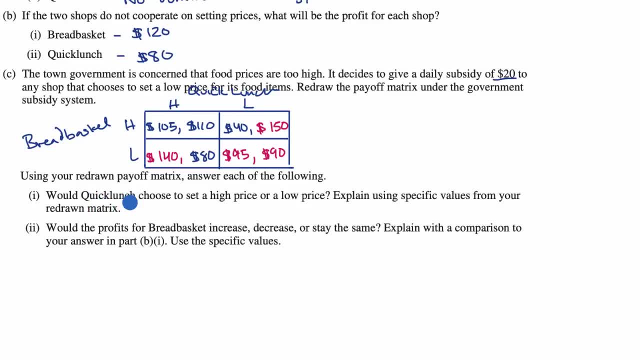 So pause the video and see if you can answer that. All right, so we're going to look at Quick Lunch now And we could do the same type of analysis to see if they have a dominant strategy. We could say, okay, if Breadbasket goes high, goes high. 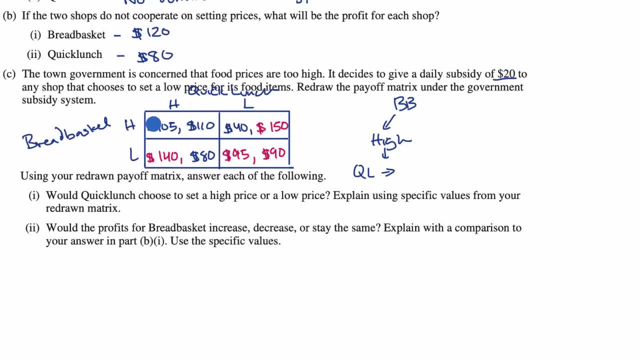 what is Quick Lunch going to do? So if Breadbasket goes high now, in this situation, Quick Lunch will either go high and make $110, or it could go low and make 150.. So if Breadbasket goes high and make $110, or it could go low and make 150,. 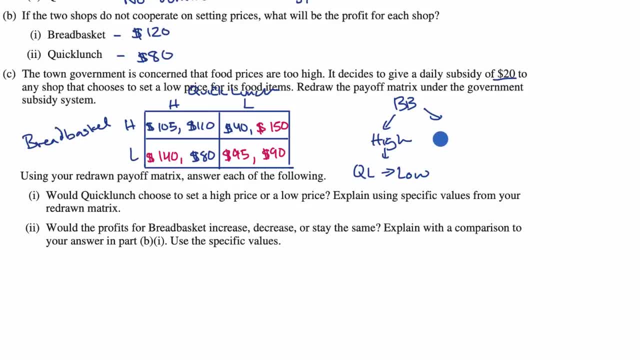 so Quick Lunch is going to go low in this situation. And if Breadbasket goes low, Quick Lunch can make $80 if it goes high, or it could make $90 if it goes low. So once again, Quick Lunch is going to go low. 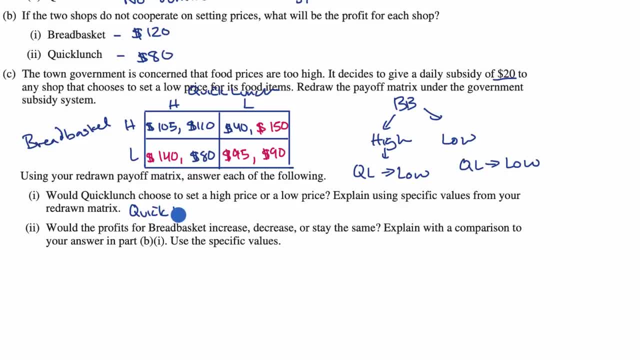 So Quick Lunch. Quick Lunch now has dominant, dominant strategy for low price. For low price, And I could try to explain this out: If Breadbasket goes high, I'll write it out here. Normally you have a little book to write this in. 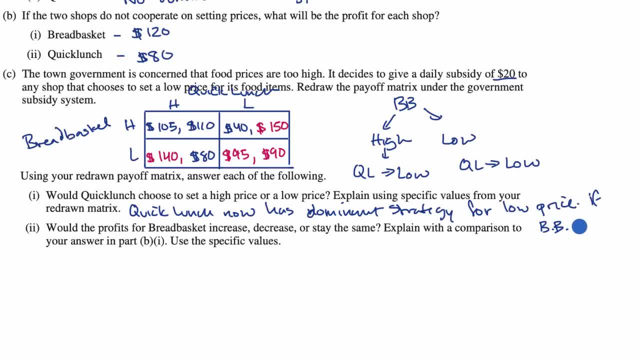 but if Bread- I'll abbreviate Breadbasket- goes high, Quick Lunch is rational to make $150 instead of 110.. Quick Lunch would want to make $150 versus 110 by going low. If if Breadbasket goes low, goes low. 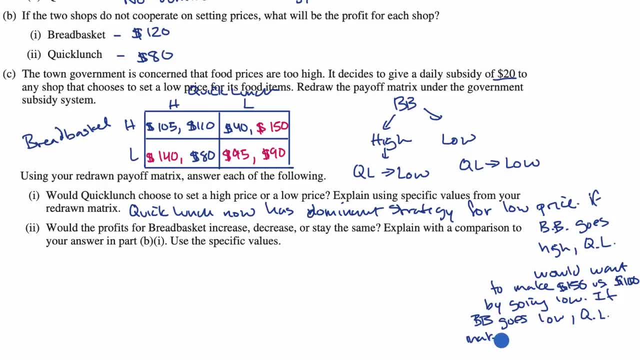 Quick Lunch makes makes $90 versus versus $80 by going low, All right. Would the profits for Breadbasket increase, decrease or stay the same? Explain with a comparison to your answer in part B1.. Use specific values, So before subsidy. 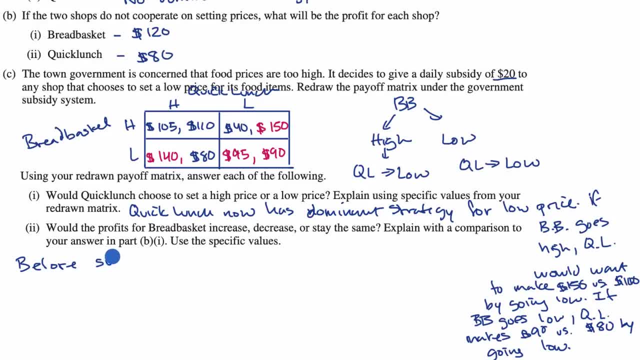 actually pause this video and try to do this as well. Heh Before subsidy: oh, now we'll do it together. Before subsidy: Quick Lunch, or I should say, Bread Basket. Bread Basket was making and we have it up here. 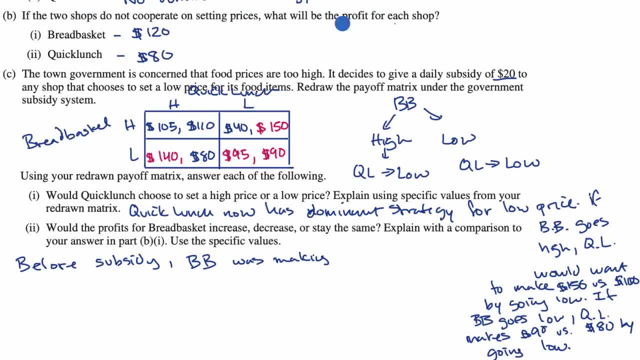 So if the two shops do not cooperate on setting prices, what will be the profit of each shop? We saw Bread Basket would make $120, because that was that Nash equilibrium state After subsidy after subsidy. so let's look at it: we still have. 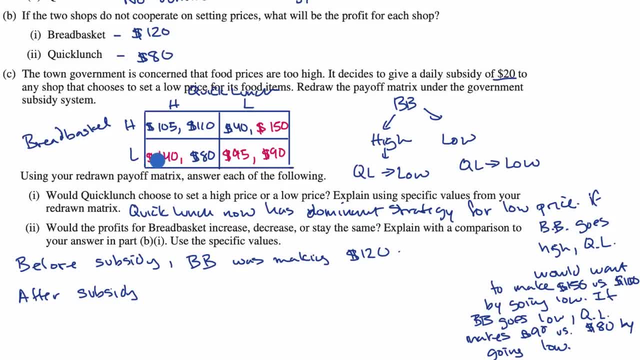 Bread Basket still has a dominant strategy to go low, because if Quick Lunch goes high, Bread Basket would wanna make the 140 instead of 105, and if Quick Lunch goes low, Bread Basket would wanna make 95 instead of 40. But now they both have a dominant strategy for going low.